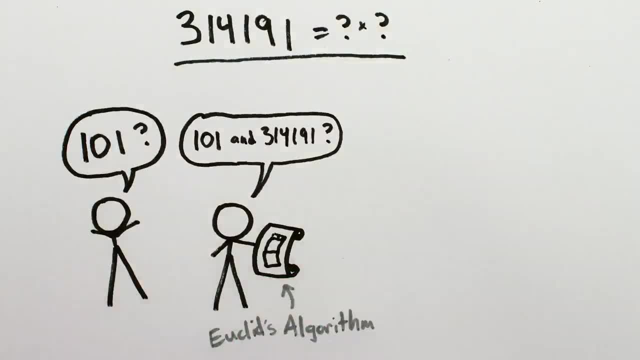 check to see if 101 shares a factor with 314,191.. And it doesn't. So our goal is to find the special power p, which is the number 314,191,, and the factor 314,191,, which is the number 314,191. 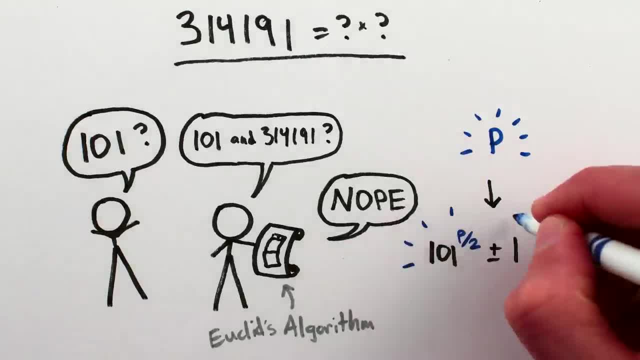 So our goal is to find the special power p, which is the number 314,191,, and the factor 314,191,, for which 101 to the p over 2 plus or minus 1 is a better guess for a number that shares factors. 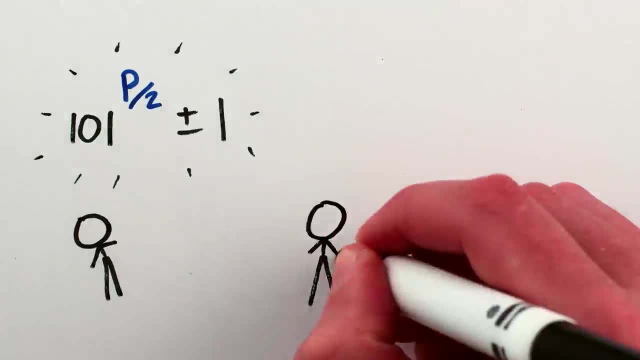 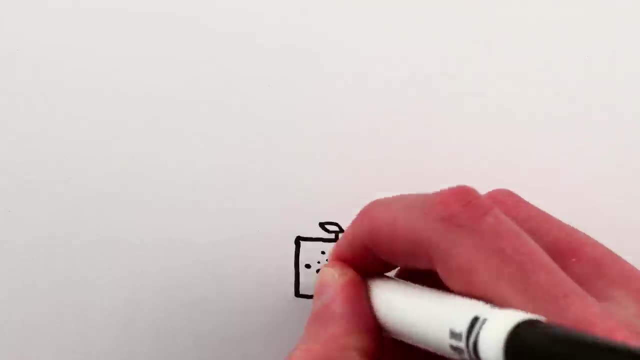 with 314,191.. To do this, we need to find the number p such that 101 to the p is one more than a multiple of 314,191.. This is where we use my quantum computer, which can raise 101 to any. 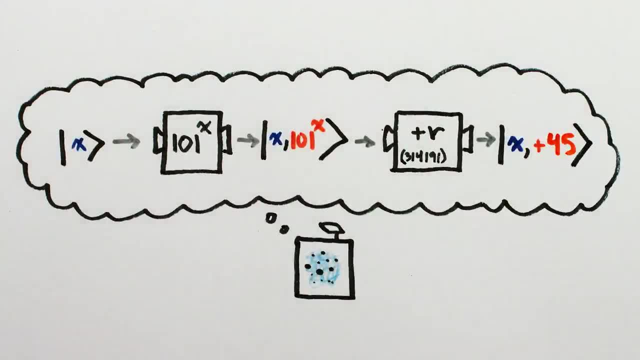 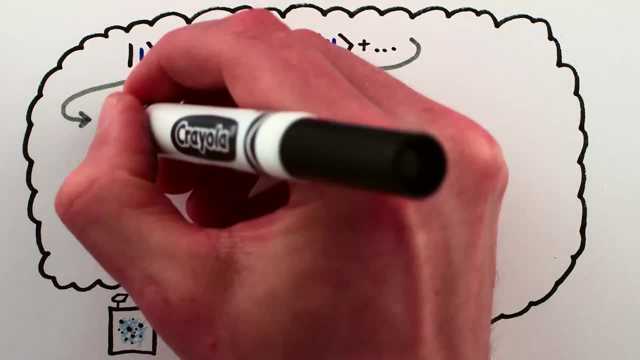 power and calculate how much more that power is than a multiple of 314,191.. If we start with a superposition of all the numbers up to 314,191, then the quantum computation we'll give us the superposition of 101, plus 101 squared, plus 101 cubed, and so on. 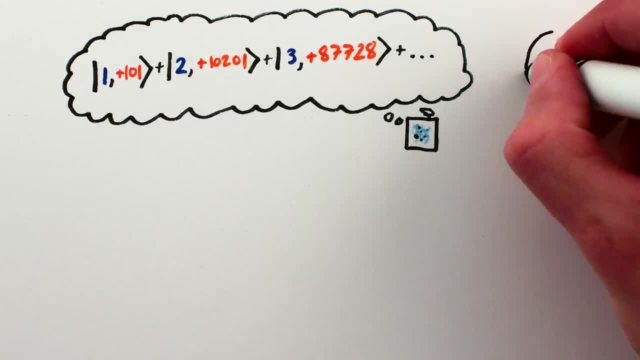 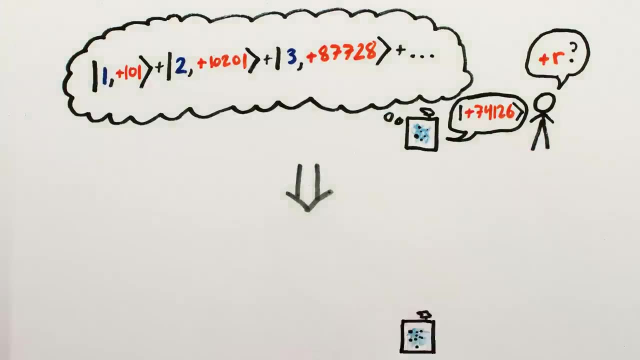 and then the superposition of the remainders. So we measure just the state of the remainders and we'll get one remainder as an output, say 74,126, from which we know that the rest of the quantum state is left in a superposition of the possible powers that resulted in the remainder. 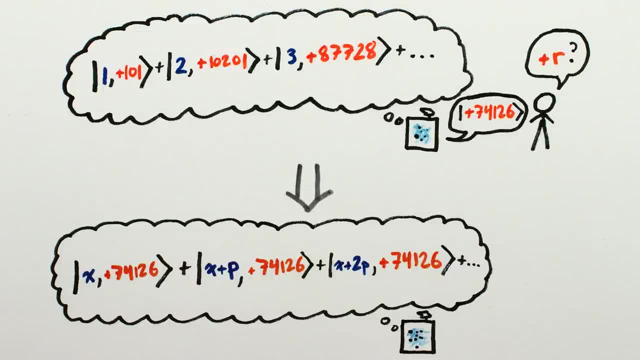 74,126, which must all be p apart from each other. I explained why in the other video, Because we're not actually dealing with particularly big numbers. I've done the calculation and can figure out how to do it, So let's do it. 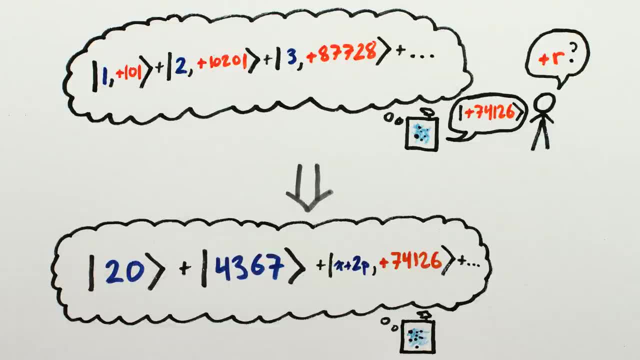 I can tell you that this would mean we had a superposition of 20, and 4367, and 8714, and so on, and the difference between them is p. But in a real situation we of course wouldn't know what the numbers in the superposition are. We just know that they're separated with 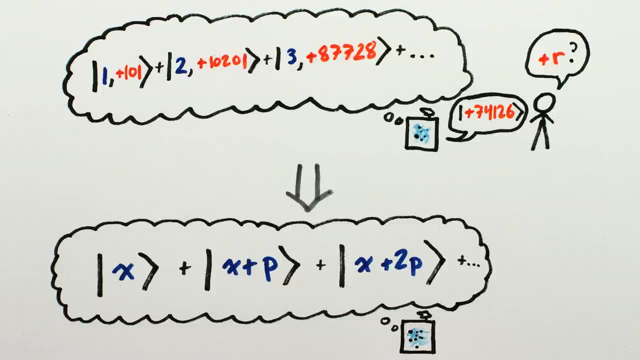 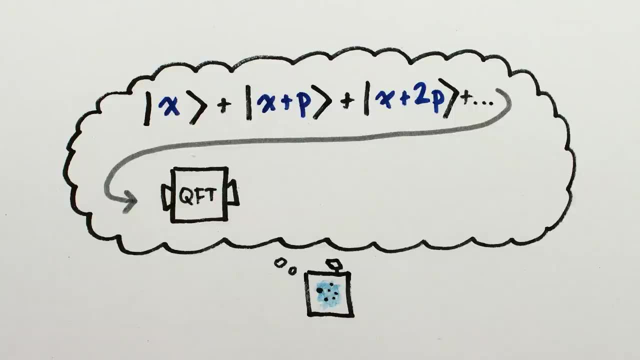 a period of p or a frequency of 1 over p, though we still don't know what p is. The next step is to put the superposition through a quantum Fourier transform, which will pick out that frequency and result in a superposition of 1 over p, plus 2 over p, plus 3 over p. 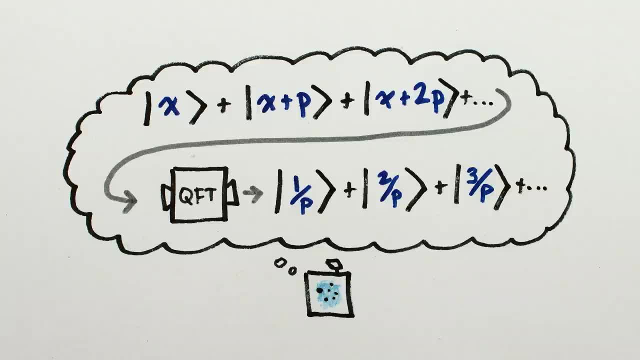 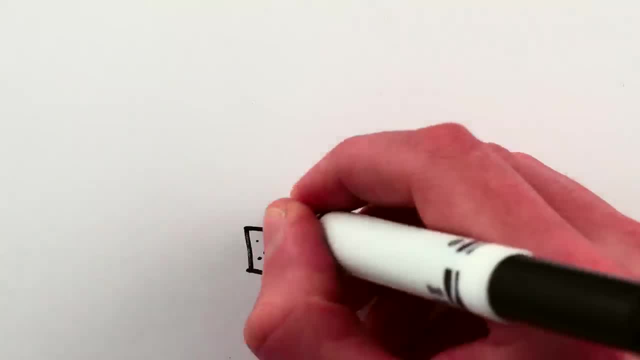 and so on. This is a part I glossed over in the main video, but for technical reasons, the quantum Fourier transform doesn't just output 1 over p, It outputs a superposition of multiples of 1 over p. Anyway, again because these are small numbers, I can tell you that we'd. 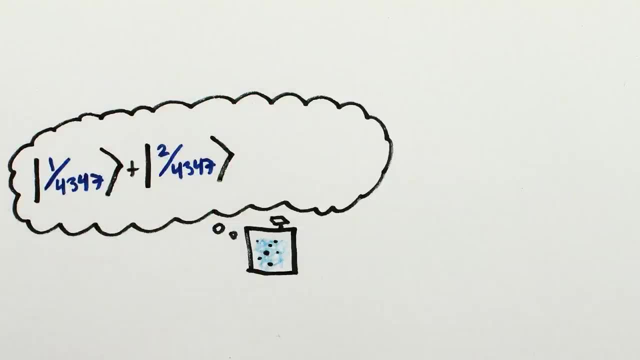 have a superposition of 1 over 4347, and 2 over 4347, and 3 over 4347, and so on. but in practice we wouldn't actually know what they were, So we'd measure the superposition. 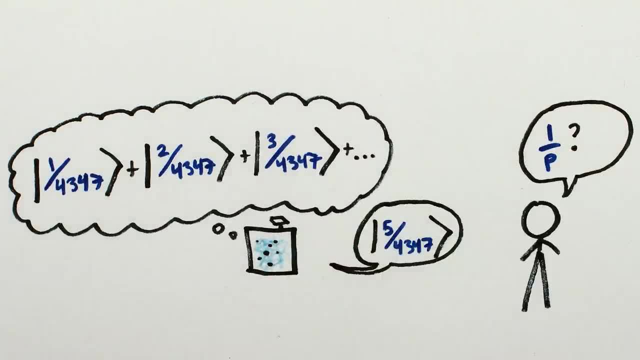 and we'd randomly get one of the values as the output, Say, for example, 5 over 4347.. And then we'd do the same thing in the other way: We'd get a superposition of 1 over 4347,. 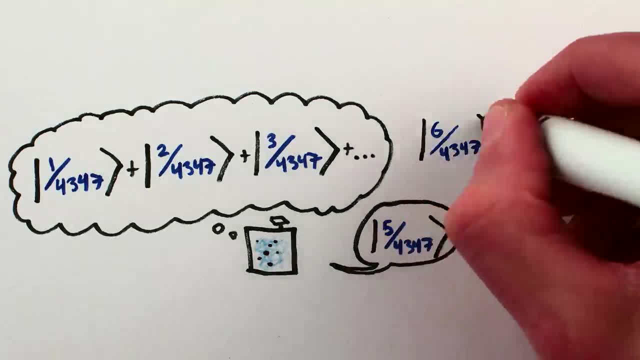 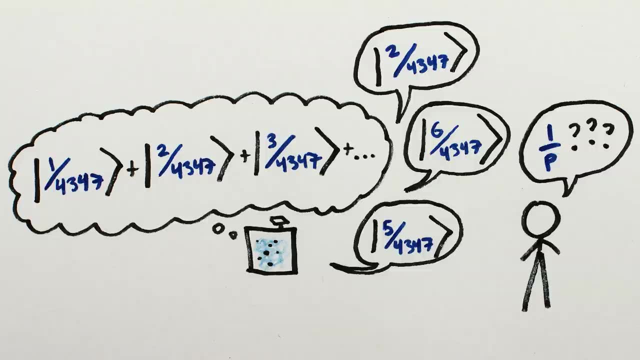 and then we'd do the calculation again and get, say, 6 over 4347, and then 2 over 4347, and so on. Pretty soon we'd be able to tell that 1 over 4347 is the common factor. 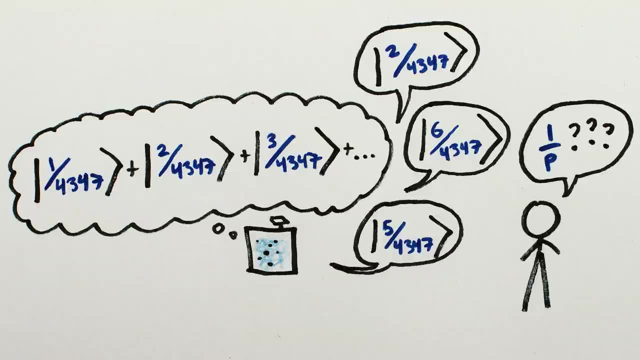 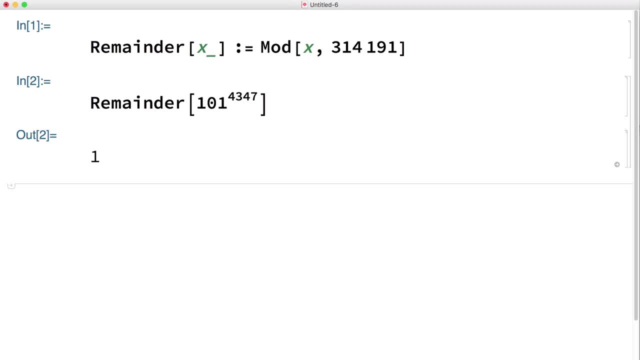 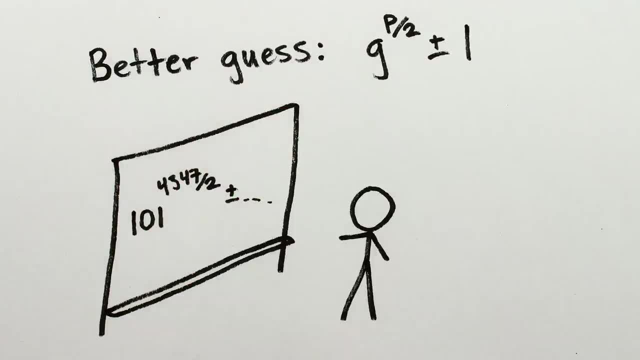 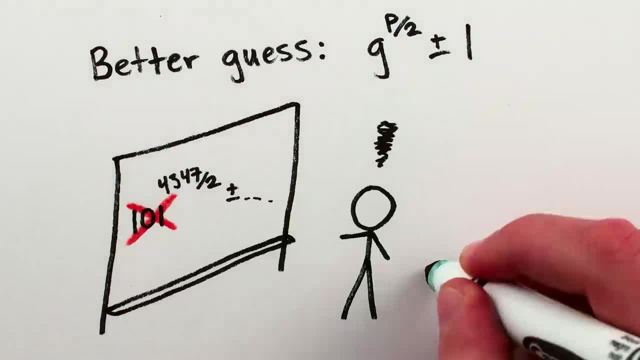 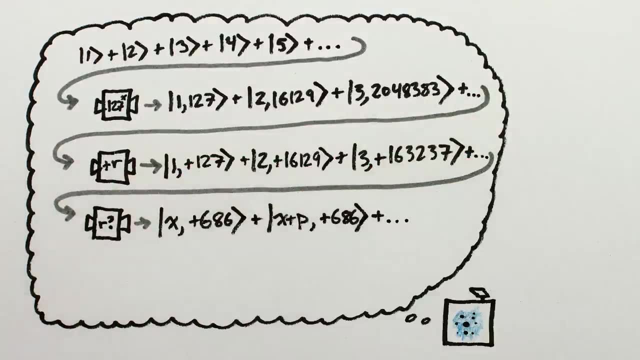 to start over. Ummm, Hmm, Let's pick, suppose another random guess and say 127.. After going through the same process of creating simultaneous superpositions, of raising 127 to all possible powers and then doing a quantum Fourier transform and so on, we'd end up. 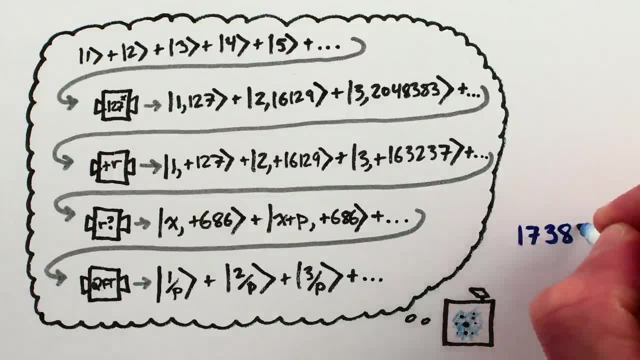 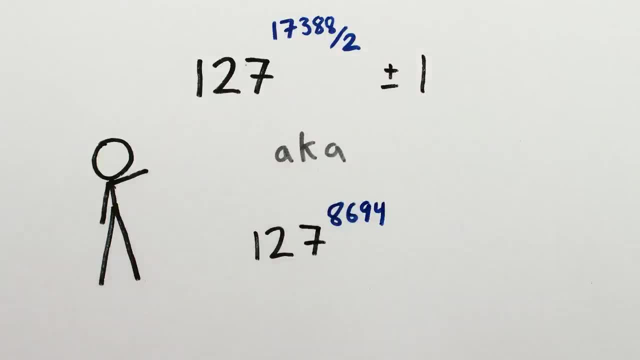 finding that that value of p corresponding to 127 is 17,388.. And so raising 127 to p over 2 gives 127 to the 8,694 plus or minus 1 for our new and improved guess of a number that shares factors with 314,191.. Using Euclid's algorithm on 314,191, 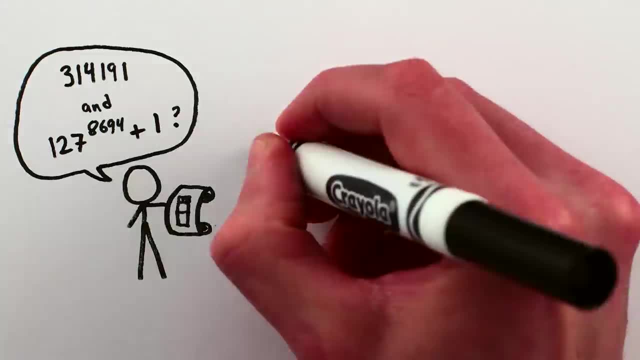 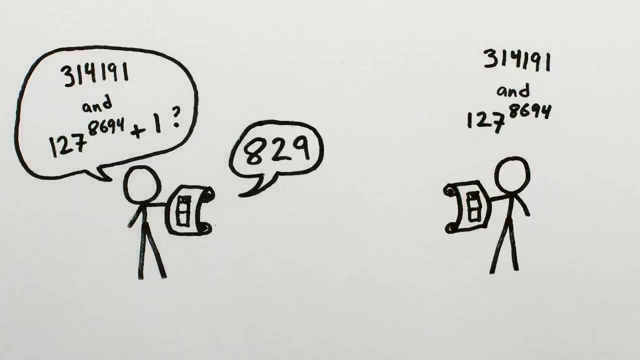 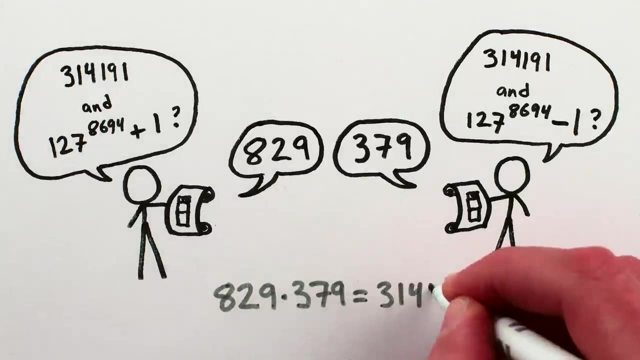 with 127 to the 8,694 plus 1, gives a common factor of 829, and using it on 314,191 with 127 to the 8,694 minus 1, gives a common factor of 379.. And 829 times 379 does indeed give us. 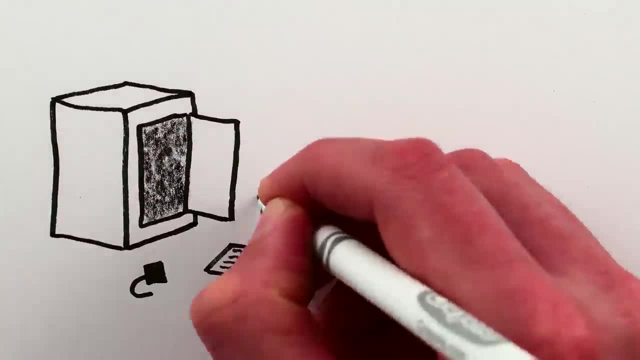 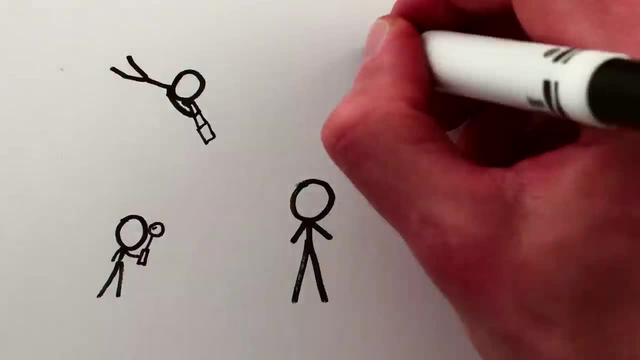 314,191.. So now we can break the encryption and you can have your pie. If you want to make sure your digital life is more secure than the bank vault in this video, then I highly recommend using a password manager to generate and securely store a long and unique